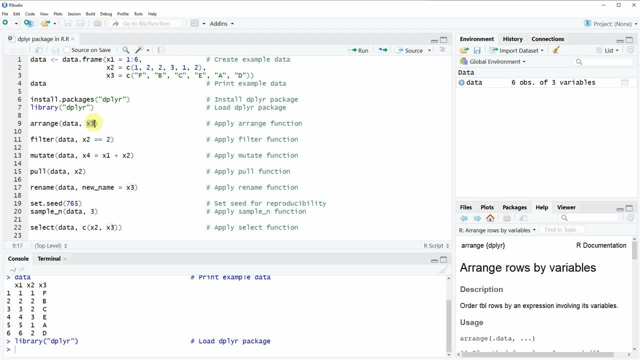 So in this case I'm going to sort our data based on the column x3.. So if you run this line of code, you will see that a new data frame appears at the bottom in the R studio console, and this time the rows of the data frame are ordered alphabetically according to the column x3.. In the next example I 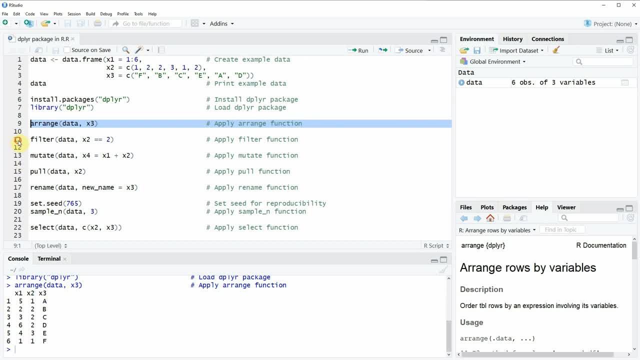 want to show you how to apply the filter function- and you can see this example in line 11 of the code- and the filter function is taking a subset of our data based on a logical condition. So in this case, in this example, I'm going to take a subset only for rows where the column x2. 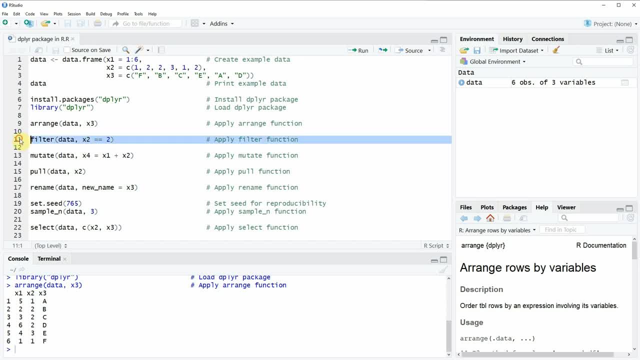 is equal to the value 2.. So if you run this line of code, you will see that another data frame is returned at the bottom in the R studio console, and this time this data frame is a subset of our data, And this subset is only containing rows where the column x2 is equal to 2.. 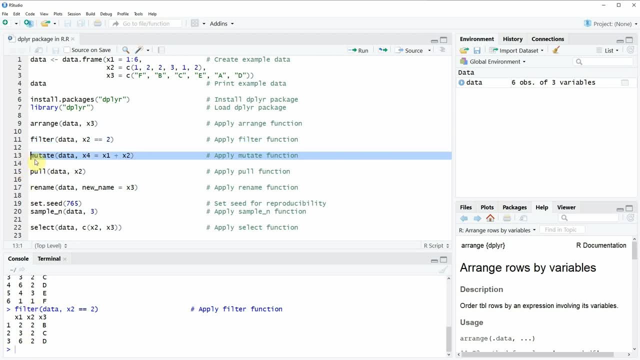 In the next example I want to show you how to apply the mutate function, and the mutate function is converting already existing variables of our data frame into a new variable. So in this example I'm going to create a new variable, x4, and this variable is going to be a new variable x4.. 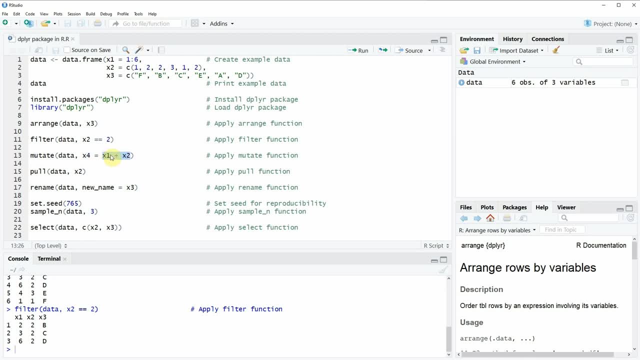 And this variable will contain the sum of our columns x1 and x2.. So if you run this line of code, you will see that another data object is appearing at the bottom in the R studio console and this data frame contains the three columns of our original data and in: 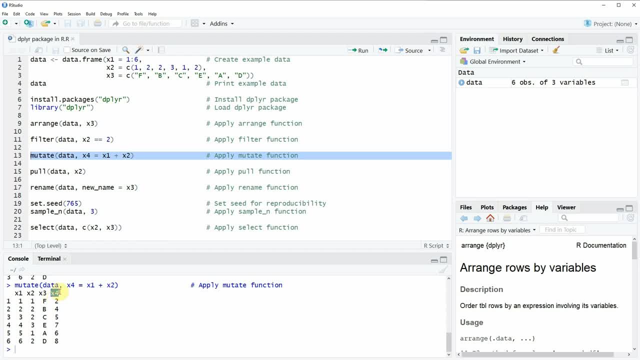 addition to that, a fourth column, x4, which is containing the sum of the columns x1 and x2.. In the next example, I want to show you how to use the pull function of the dplyr package. and the pull function is extracting one column of our data frame and converts this column into 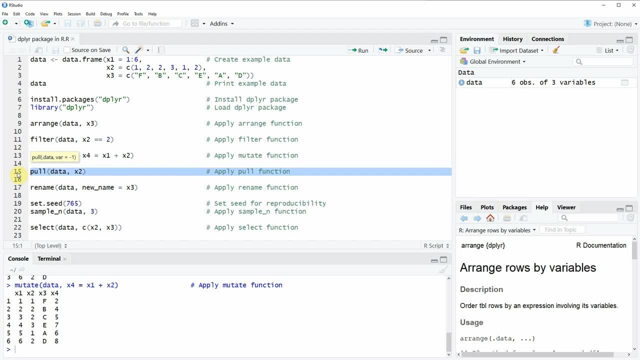 a vector. So let's assume that we want to extract the column x2 from our data frame. then we can use the code here of line 15 and if you run this line of code you will see that the values of our column x2 are the values of the column x2.. So if you run this line of code you will see that the values of our column x2 are the values of our column x2.. 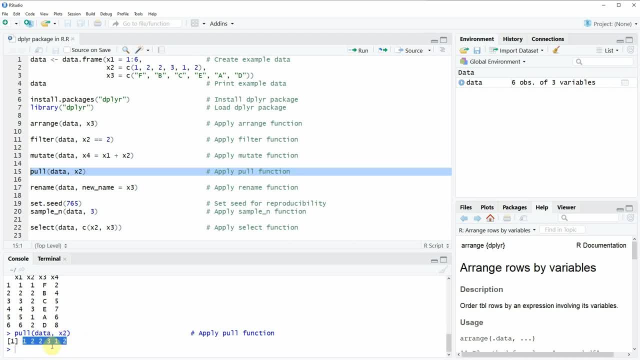 are returned to the R studio console. In the next example, in line 17, I want to show you how to use the rename function of the dplyr package. and the rename function is used to change the names of the columns of our data frame. So in this case I want to change the name of our column x3. 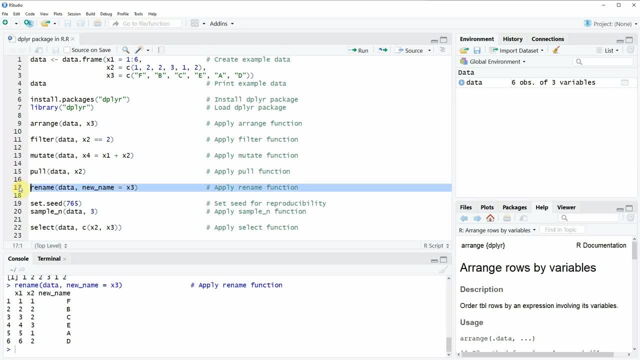 into a new name. So if you run this line of code, then you can see that the values of our column x2 are returned to the R studio console. Then you can see that this data frame here contains exactly the same values as our original data frame. 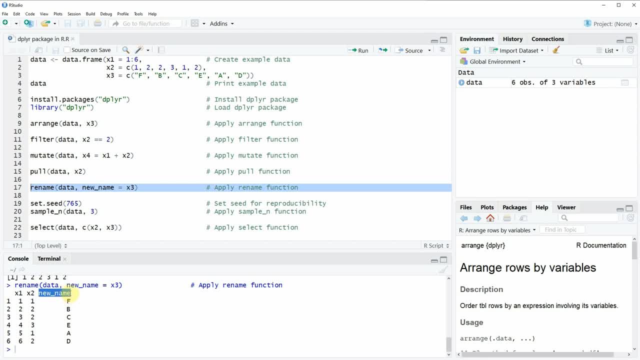 but in this case the variable x3 was renamed into the name new name. In the next example I want to show you how to use the sample n function and the sample m function is randomly taking a subsample from our original data frame. Since we are going to take a random subset of our data frame, it makes a lot of sense to set a seed. 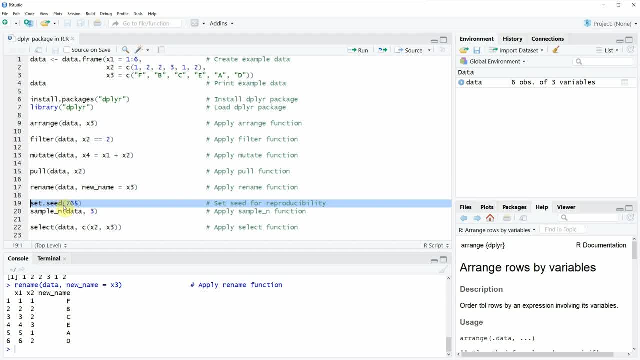 before we apply the sample n function, because this seed ensures that you can reproduce the code as I'm showing here in the video. So if you run this line of code, our seed is set to 765 and now we can run the sample n function. 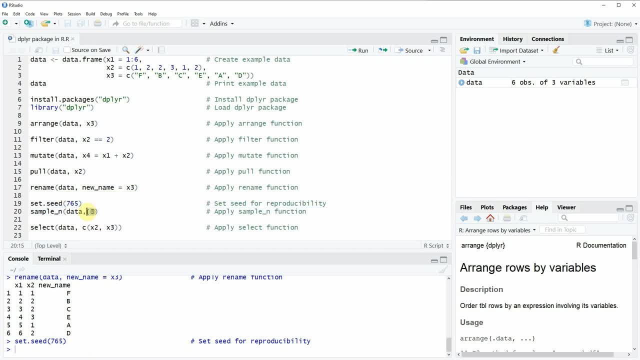 As you can see in line 20 of the code. so in this case we are specifying within the function that we want to randomly sample three rows of our original data frame. So if you run this line of code, you can see that exactly three rows of our original data frame are returned.